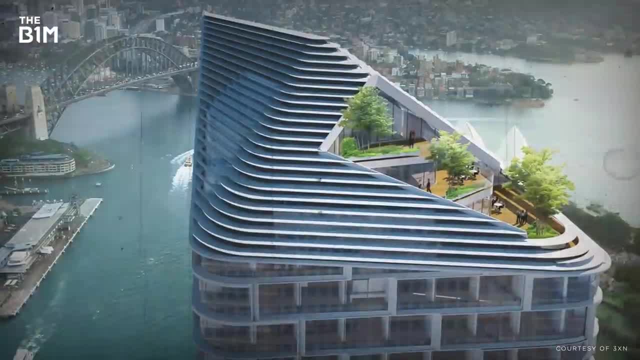 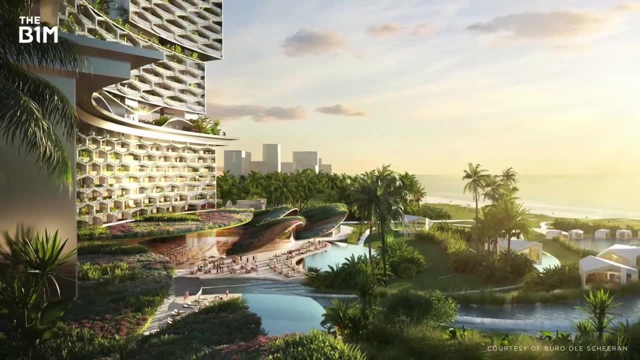 Look at almost any skyscraper that's been put forward in the last decade or so and you might notice a budding trend. They all have trees on them, and it all seemed to start with these controversial high-rises in Milan. Now, green-covered towers aren't just meant to. 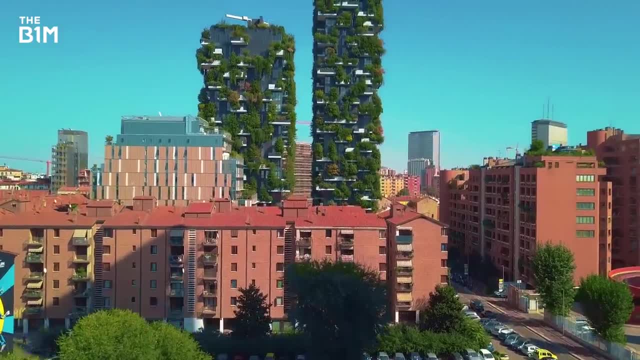 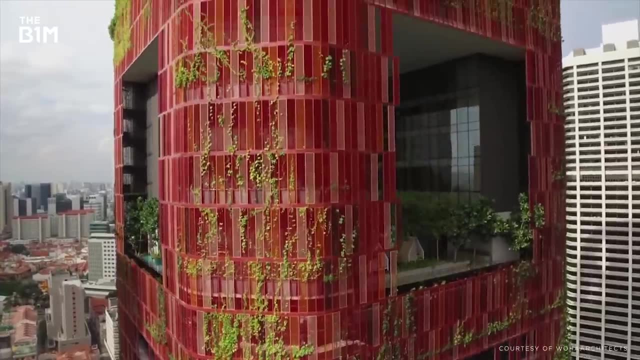 stand out like giant chia pets across drab glass and concrete skylines. Vertical forests like this aim to improve our cities by cutting CO2, providing shade, attracting wildlife and even improving our mental health. But when you take off the rose-coloured glasses, 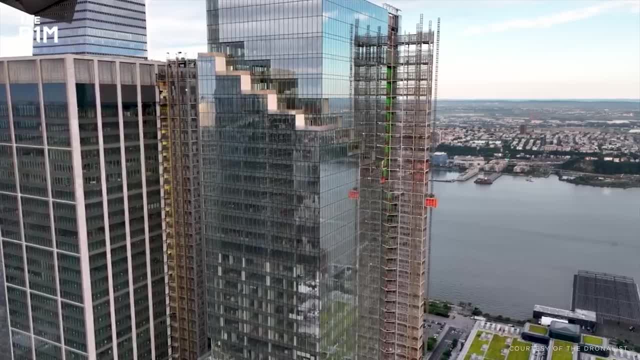 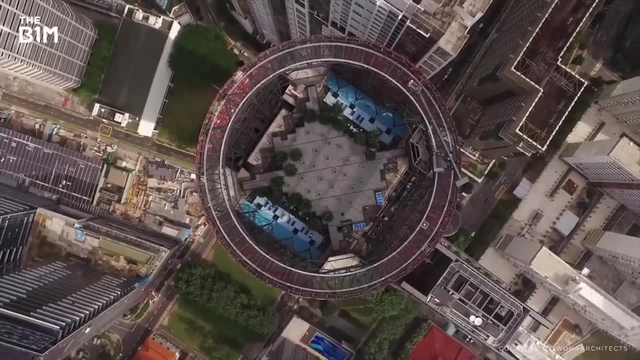 just how green are these green skyscrapers? How is vegetation even maintained so high above the ground? And if it's such a no-brainer, why doesn't every new building look like this? It's time to dig up the truth under these forests, in the sky. 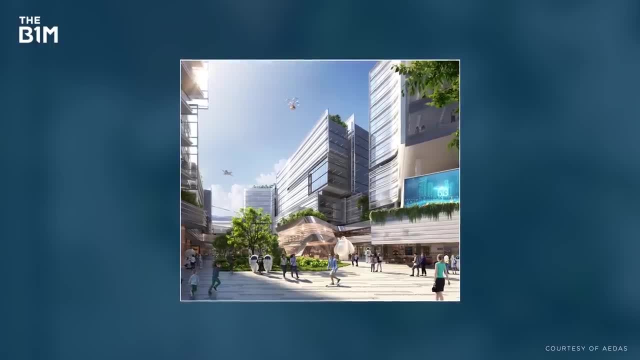 Architects: sticking trees on new building renders is becoming a bit of a thing. It's time to dig up the truth under these forests in the sky. Architects, sticking trees on new building renders is becoming a bit of a thing. It's time to dig up the truth under these forests in the sky. 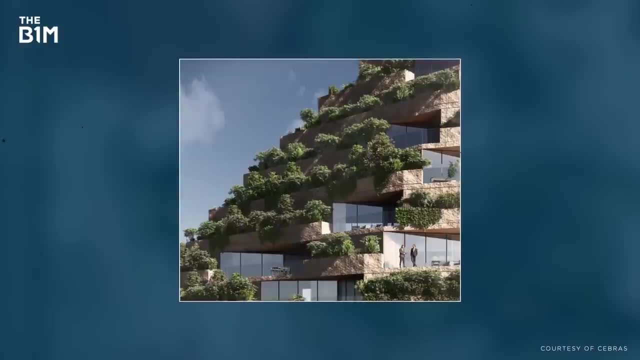 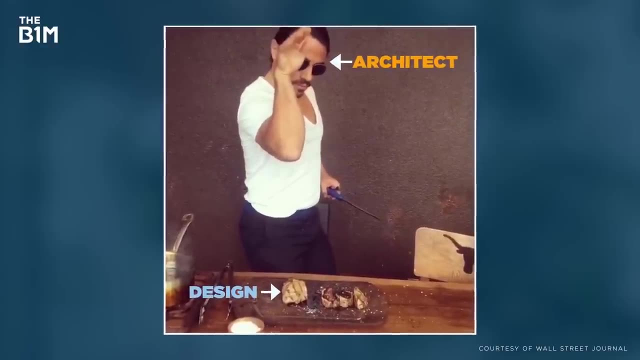 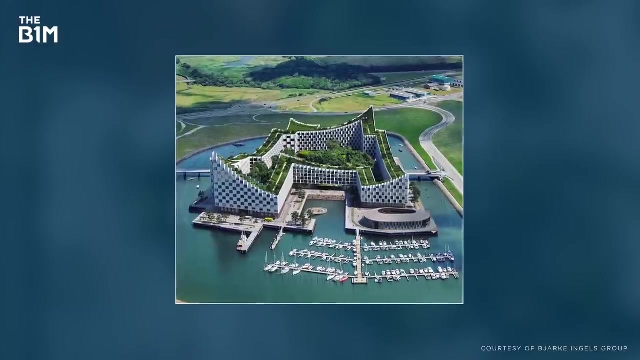 A bit of a joke. It's now so common that light-hearted suspicions of some kind of automated AI program or a senior partner sprinkling trees on projects just before things go out the door have been doing the rounds. Some question the cost and maintenance that adding trees brings versus the benefits. So is this just a shallow trick? 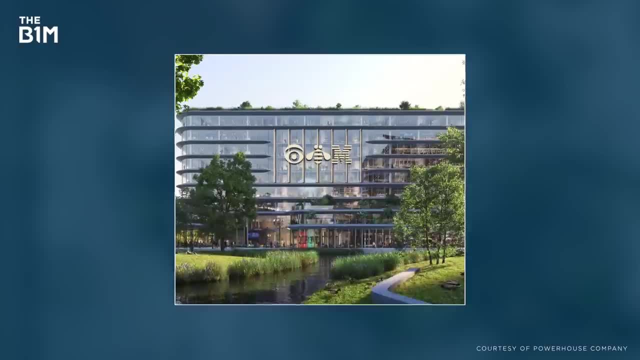 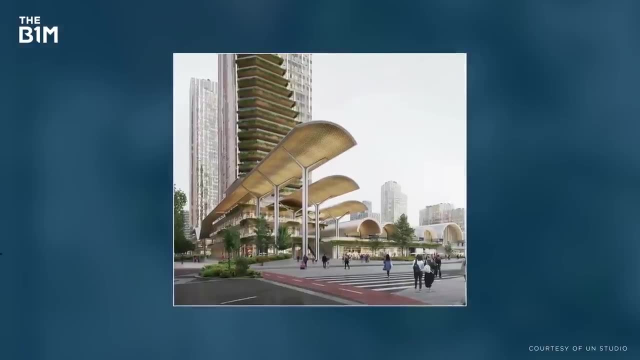 to boost social media or commercial interest in projects and make them feel sustainable, Or is there a genuinely more noble purpose? Well, to really answer that, you need some more context, and that means zooming out a bit. Walk through cities like New York. 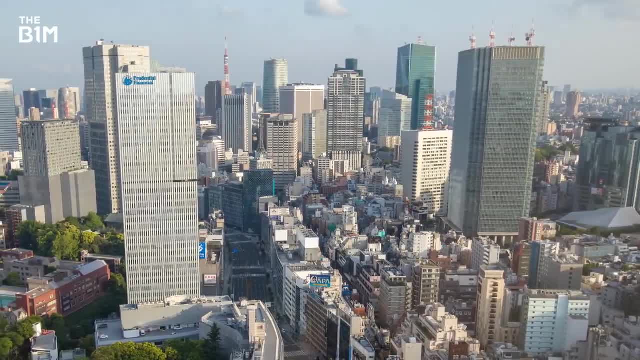 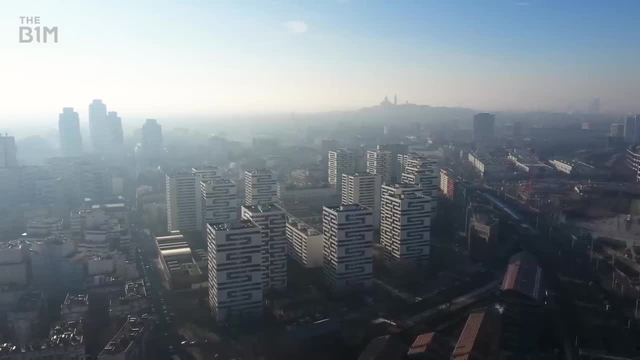 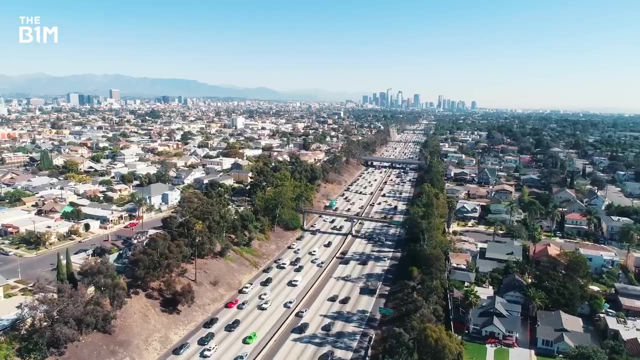 London or Tokyo and they seem massive, But compared to all of the Earth's land, built-up areas only really take up around 1% of the space. And yet our urban areas are responsible for around 70% of global CO2 emissions, and skyscrapers and cars are among the main culprits. 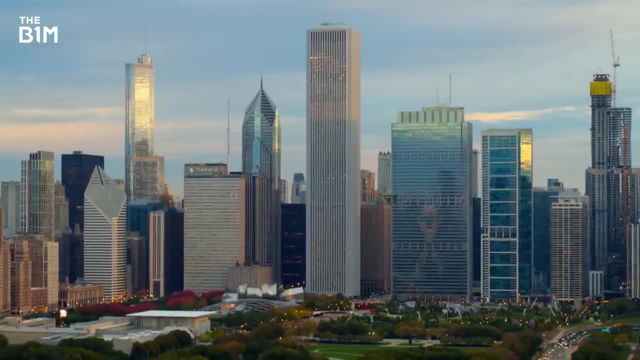 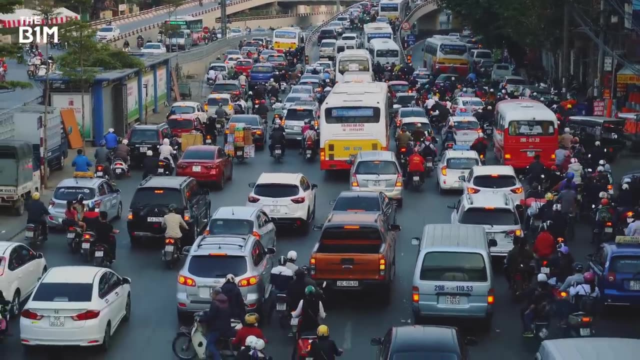 While many of us may not realise it. if we really want to tackle climate change, it's kind of essential that we build and use our buildings, cities and transport systems in a much more sustainable way: Expanded public transport, better building insulation, renewable power sources like solar. 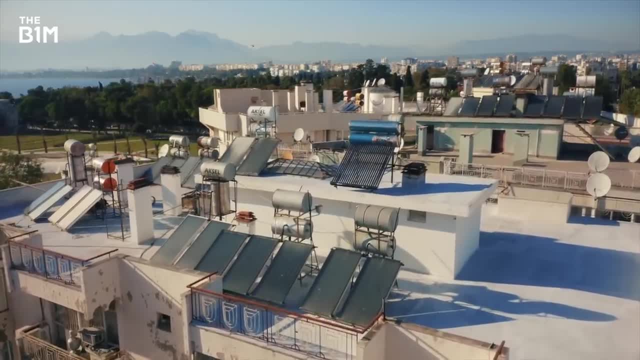 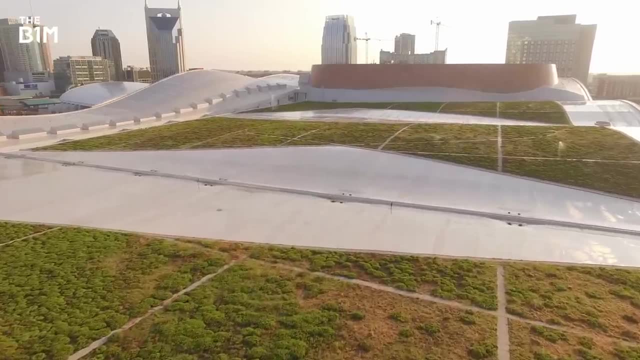 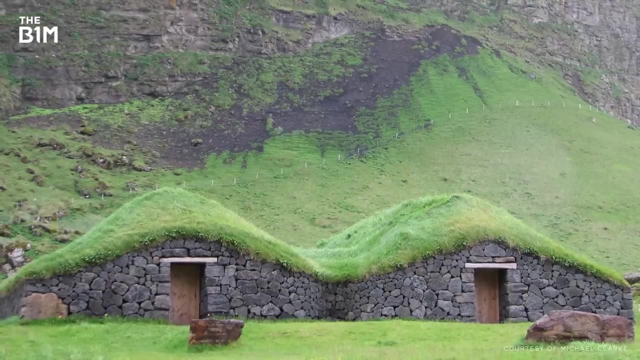 and smart temperature systems can all help with this, And so can greenery. So how exactly did this trend plant its roots? Well, it's not entirely new, but while there have been green roofs and garden roofs for centuries, we can kind of pinpoint the start of the current trend to one little spark. 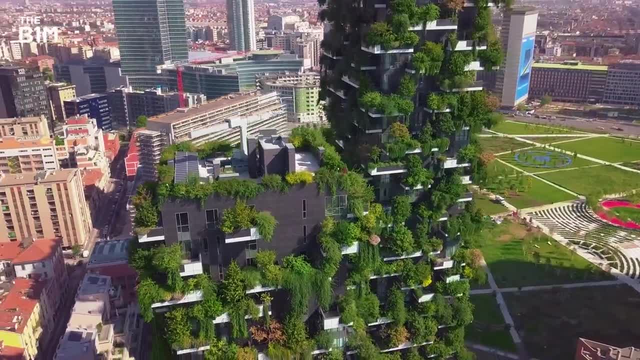 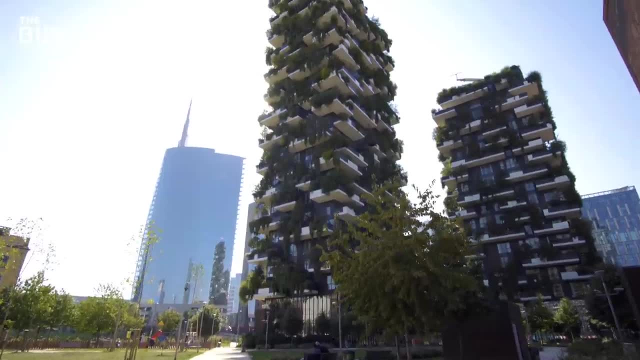 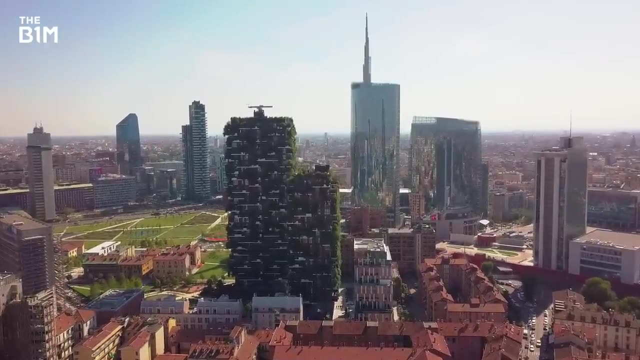 over in Malaysia. This is Bosco Verticale or Vertical Forest, which completed back in 2014.. Designed by Italian architect Stefano Baueri, the two high-rise towers are covered in thousands of trees and shrubs and stand 112 and 80 metres tall respectively. More on how they engineered. 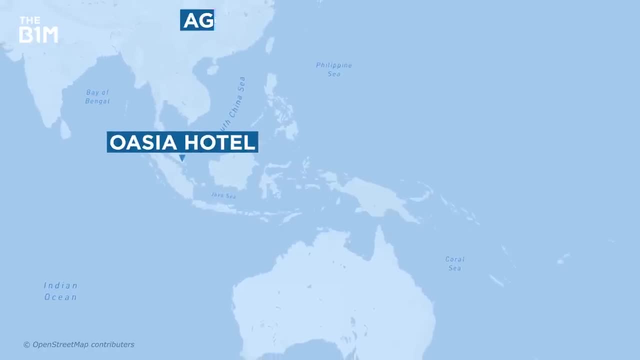 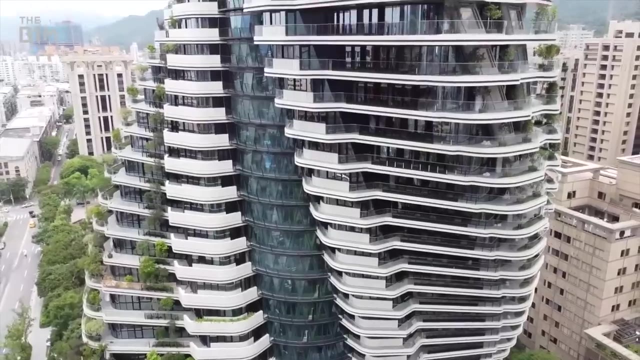 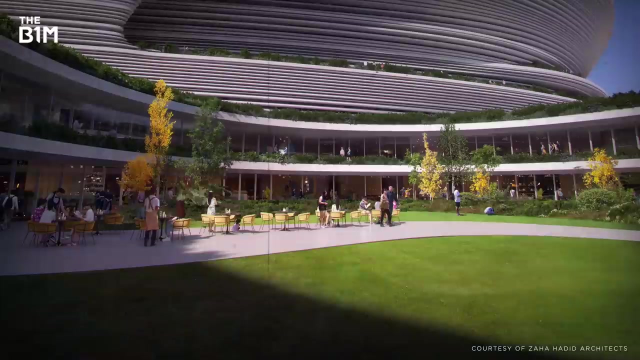 all that in a bit. Since this building came on the scene, similar structures have popped up all over the world. There's one central park in Sydney, Agara Garden Tower in Taipei and the Oase Hotel downtown in Singapore. In fact, the tree thing really is happening everywhere. 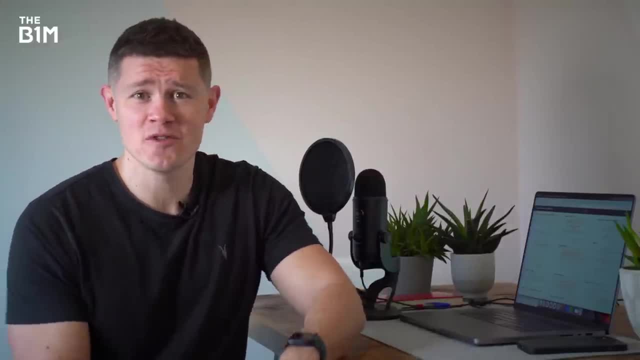 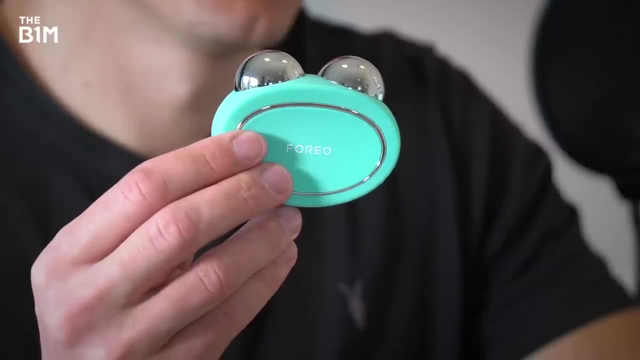 Now I know what you're thinking. Why have you interrupted a video about engineering with your face? Well, rather like those tree-covered buildings, I also require a little bit of work to look good, and that is where this little beauty comes in. 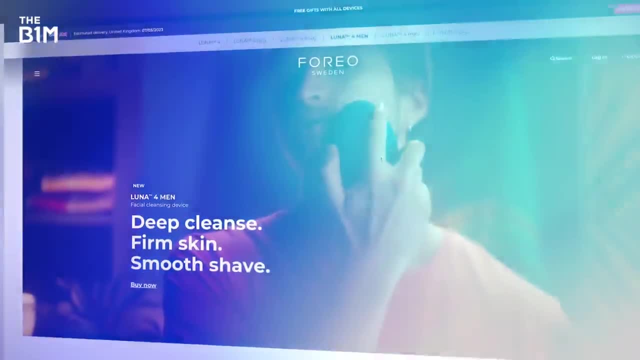 Yes, we're doing this. Stay with me for the ride. It's made by FOREO, a delightful Swedish brand that's putting beauty and tech together, And if you're interested in learning more about this brand, please check out the video above. 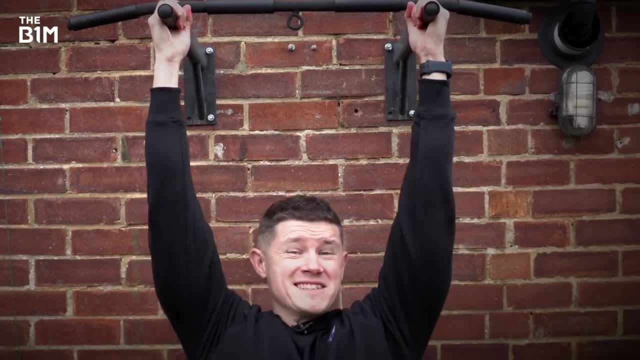 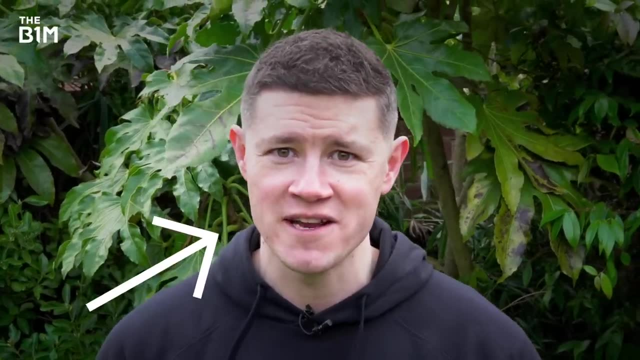 Now, while I never miss back day, there's one part of my body that doesn't always get my workout routine and, as such, ends up looking a little less buff. That's right, my face- Ironically, the part of me that most of you actually see. 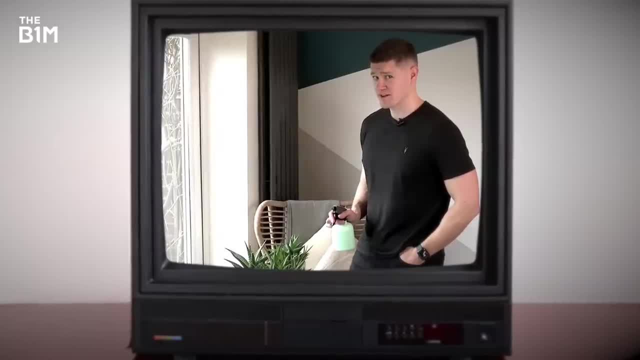 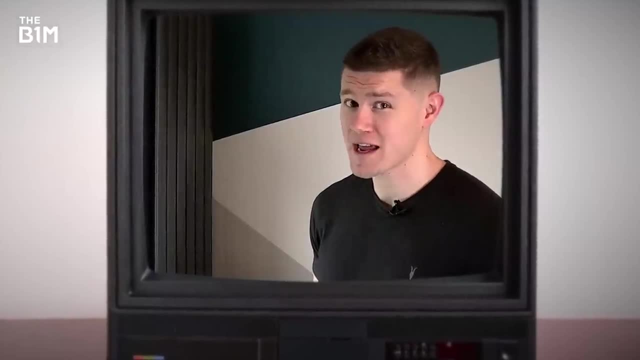 Don't go anywhere. here comes the big reveal. Spoiler alert: guys like to look good too, especially international YouTubers, And the ones that tell you they don't are probably lying. That's where Bear by Forio comes in. 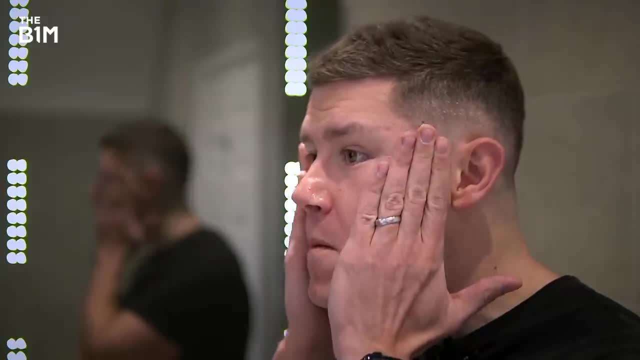 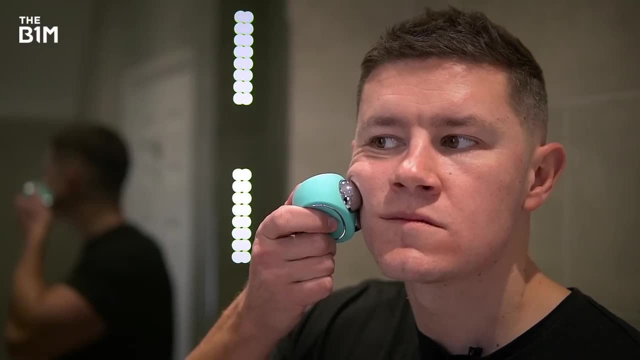 It uses some very clever tech to give you an instant facelift from your home. Basically, low voltage electrical currents called microcurrents help to naturally contour and lift your skin and facial muscles. Think of it like an incline bench press, but for your face. 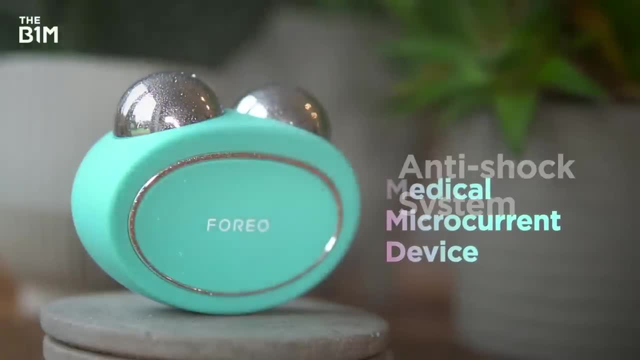 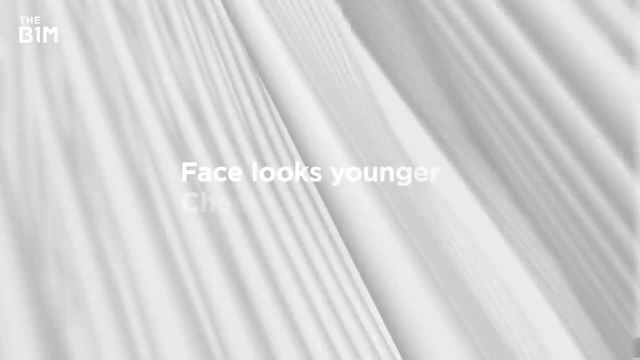 Bear is the world's first FDA cleared medical microcurrent device with an anti-shock system. It uses pulsations to energise and firm the muscles in your face and neck. 95% of people using it say their face looks younger and that their cheekbones look younger. 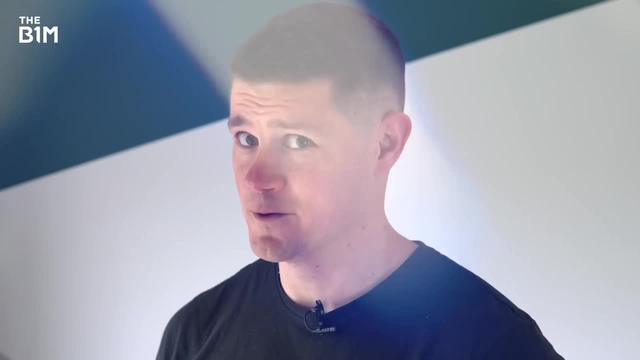 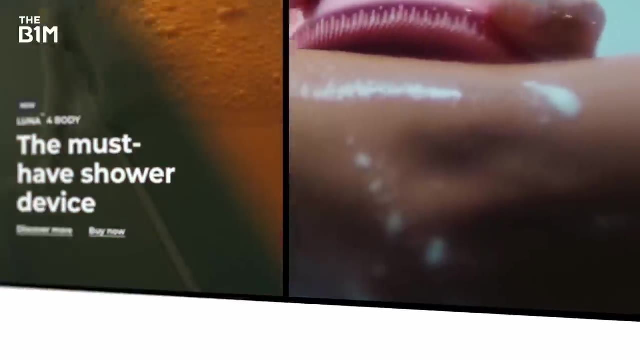 and that their cheekbones look more lifted. You should have seen me before Now. Forio has tons of facial devices, but Bear is one of the coolest gadgets out there. So if you're worried about finding something for an anniversary or birthday, it makes the. 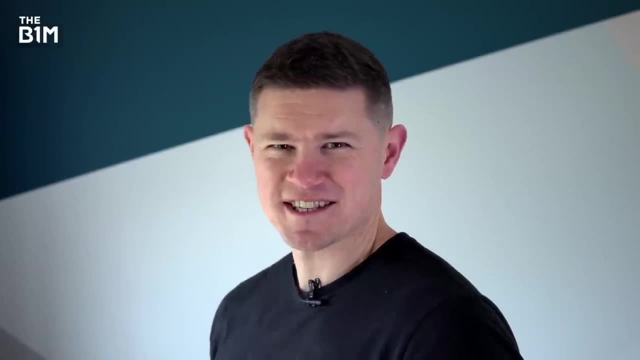 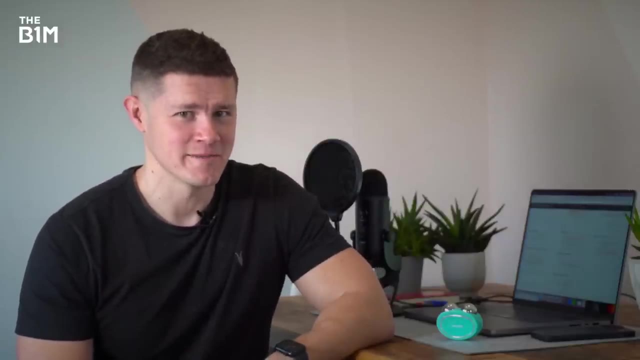 perfect gift for your significant other, Like giving them a little secret weapon to looking good. You can learn more about the Bear at the link below. but that's enough branching out. Let's get back to those trees Now. while Bosco Verticale may be considered very influential at the time of its construction, 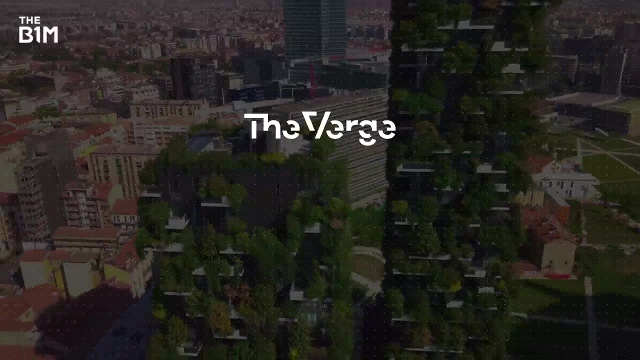 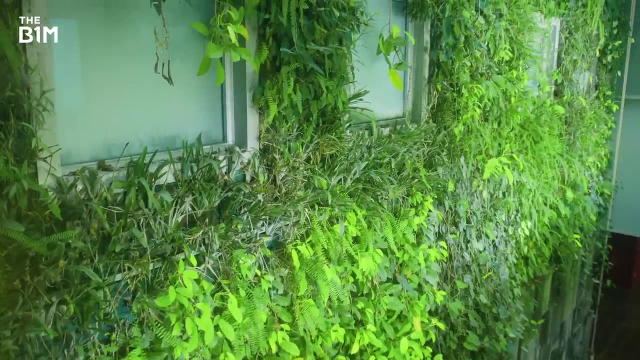 it wasn't exactly popular. Critics thought the idea was too ambitious and that nature at such high altitudes simply wouldn't work. Fast forward to today, and its greenery is clearly thriving, Although, as you might have guessed, building and maintaining structures like this isn't. 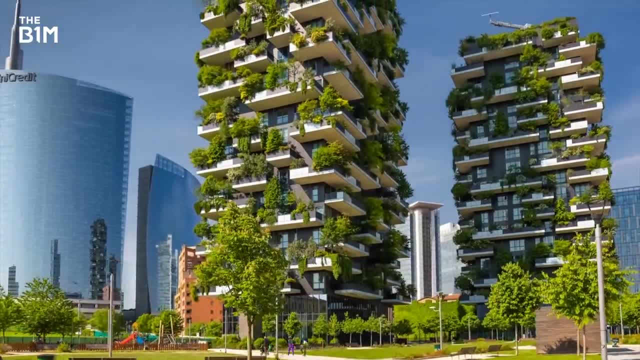 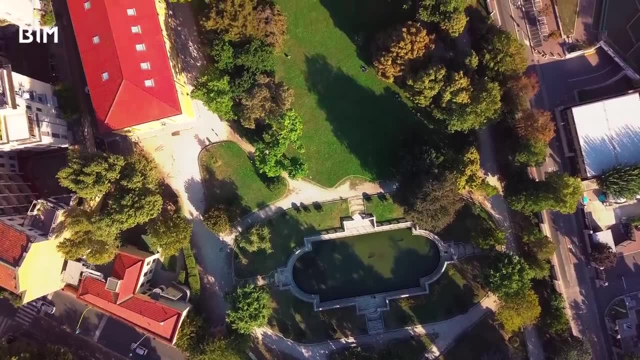 all sunshine and daisies. The residential towers themselves may have been simple in design, but the added greenery created entirely new challenges. Before construction started, architects studied vegetation in the area. They found that it was a good idea to build a greenery in the area. 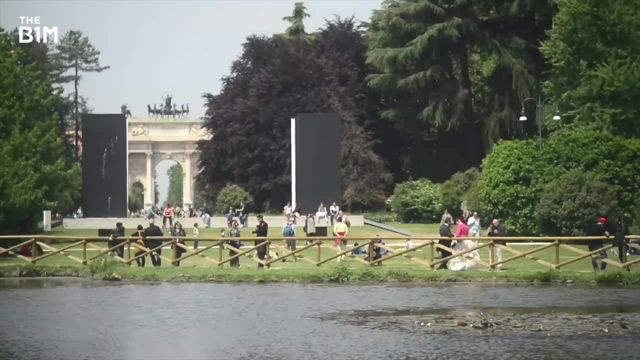 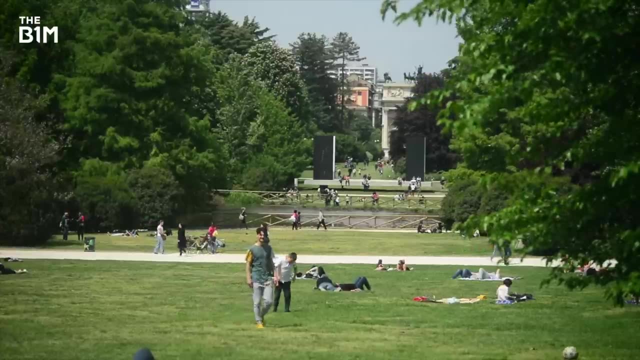 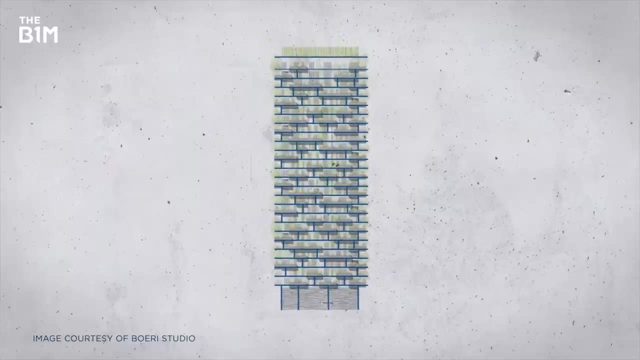 They looked at vegetation in the area, consulted experts in the field and looked at average weather conditions. They then tested and monitored plants in high wind situations before picking and choosing what vegetation could be planted and where. Structurally, the project team used a customised framework and scaffolding layout. 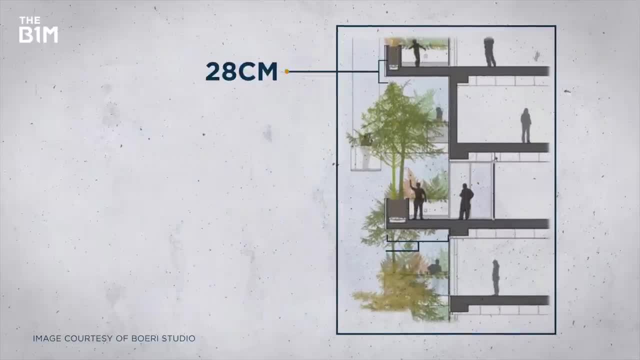 Each of the concrete balconies are 28cm thick, extend 3.35m outwards in an irregular arrangement and are reinforced with steel to carry the extra load of vegetation. Once the building's superstructure was complete, the largest and most vulnerable trees were 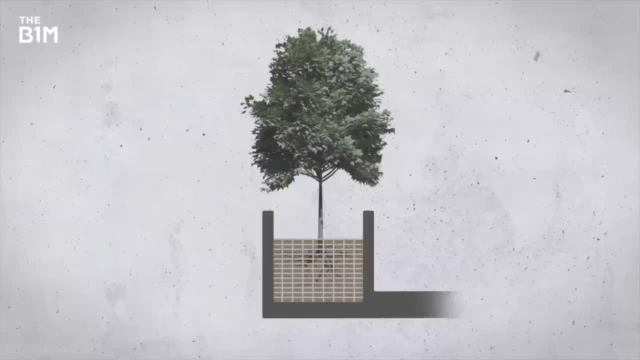 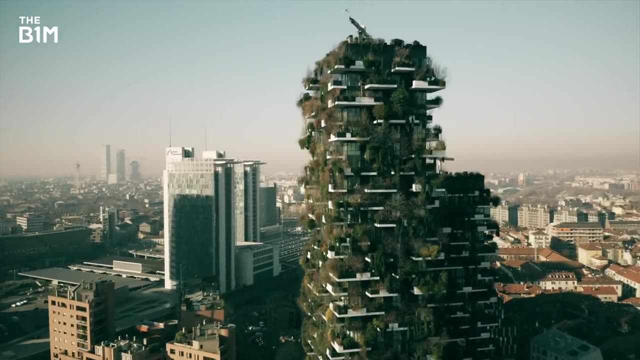 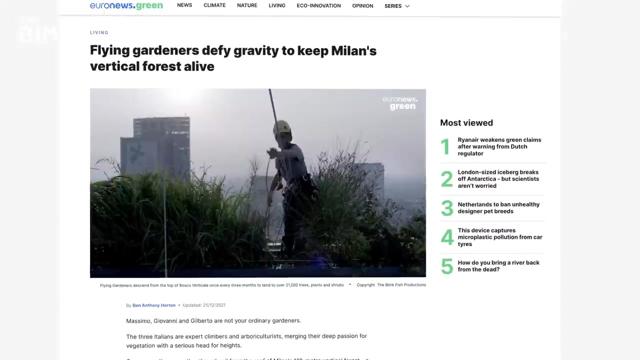 restrained within steel safety cages. Other plants sit inside concrete containers that range in size. Since its completion, the building's vegetation is regularly monitored and maintained. A unique centralised irrigation system uses recycled rainwater and keeps the plants nourished. There's also a crew of specialised arborists, dubbed the Flying Gardeners, that hang down. 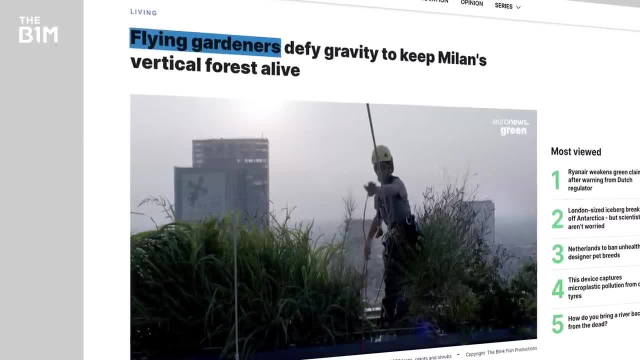 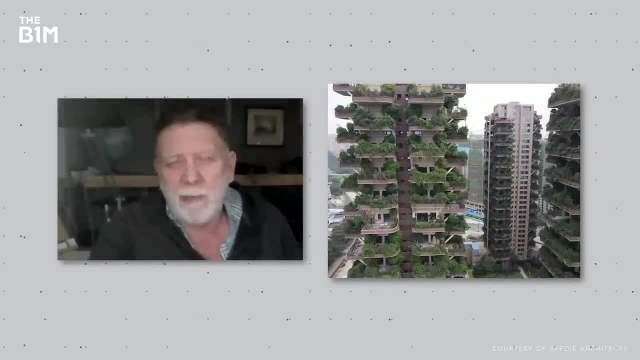 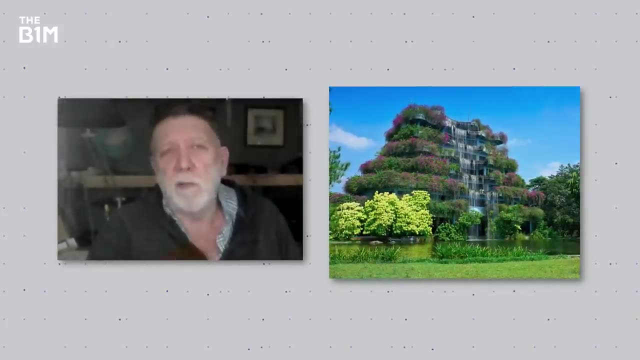 the side of the buildings every few months. There's usually a piped system that does that. There are a few passive systems where the water cascades down through it, but most of them you've got a pipe system which is pumped and controlled by computers so that the amount 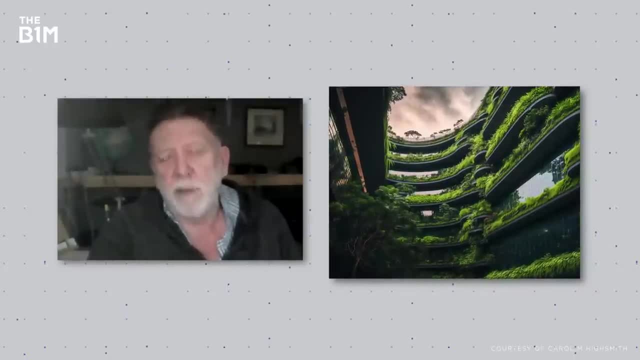 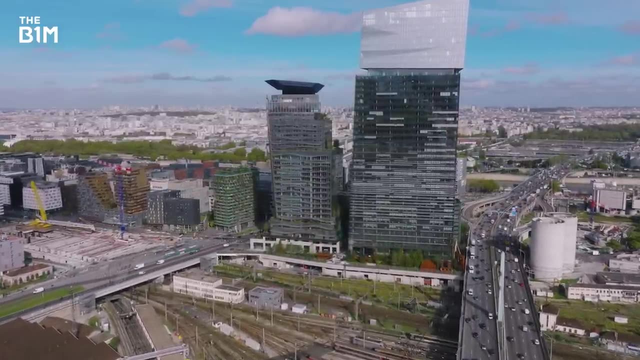 of water that gets to the plants is correct for the plants and for the climate, and so on. Now, while the tree-covered building trend has continued to grow all over the world, there's more to it than just creating some very nice looking architecture. 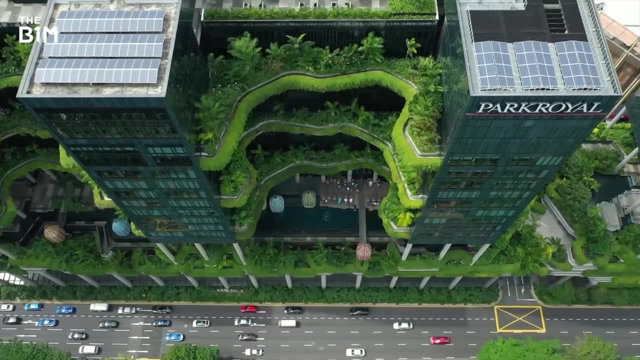 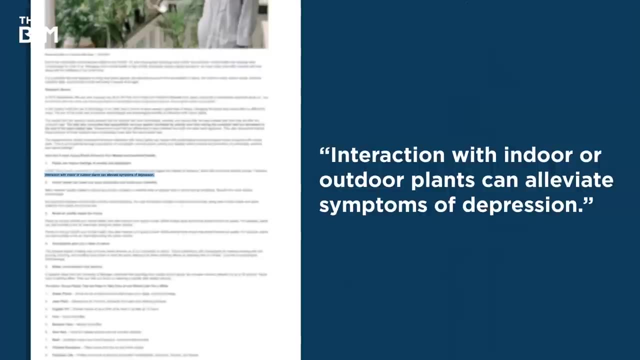 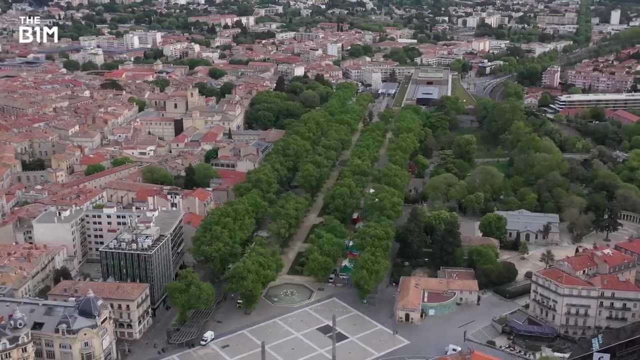 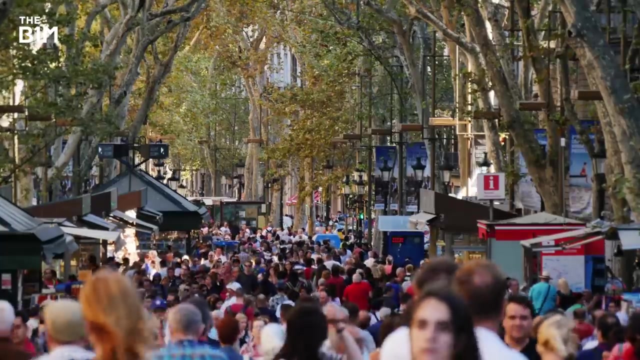 For one, plants are known to have positive impacts on mental health. One study found that seeing vertical vegetation within a city led to lower stress levels and less negative emotions, as compared to areas without greenery. The other big one is summer cooling. So if you've got soil and vegetation on anywhere actually in the heat of summer, you're getting 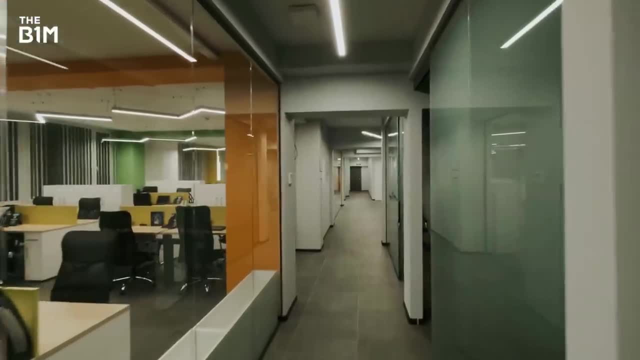 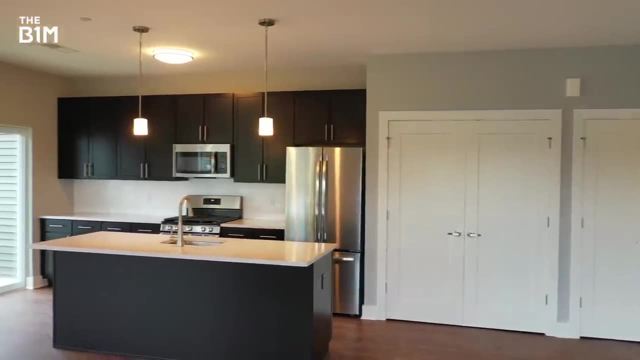 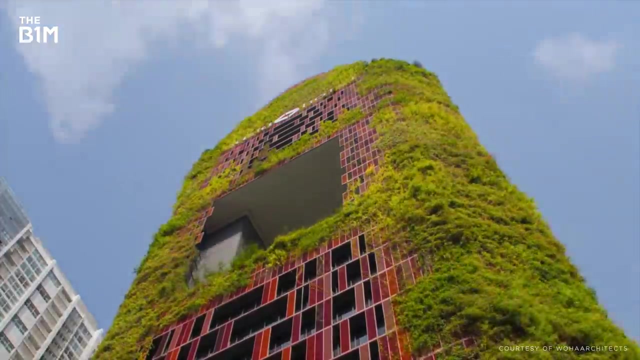 shade and evaporative cooling And so that's reducing air conditioning demands. So that can be a big plus because that can save electricity consumption. After about 20 to 30 years of that reduced use in your typical building, things start to really add up in terms of cost savings and overall carbon footprint. 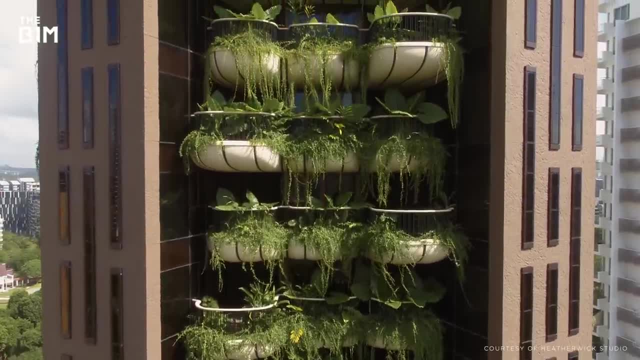 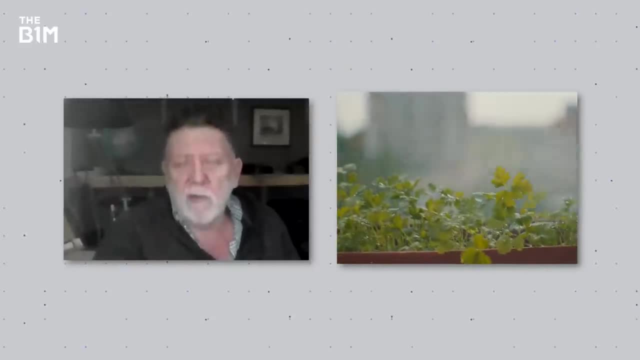 And the benefits don't stop there. The other big one is biodiversity. We know that by choosing the right plants in the right combinations, we can really make the urban area more attractive to people, And it's a big plus. It's a big, big plus. 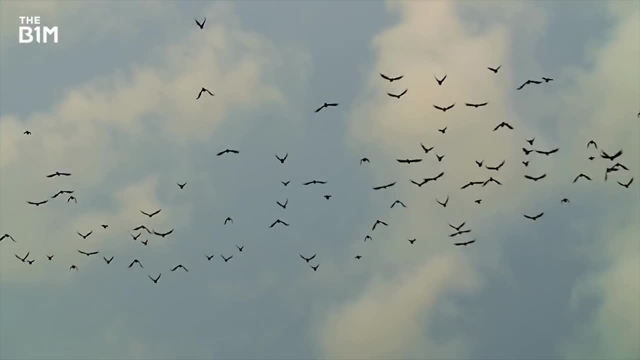 It's a big, big plus. It's a big, big plus, I think we can really move to wildlife birds, especially like this. A lot of birds can feed and nest in these features. Ever since its construction, Bosco Verticale has exploded with wildlife. 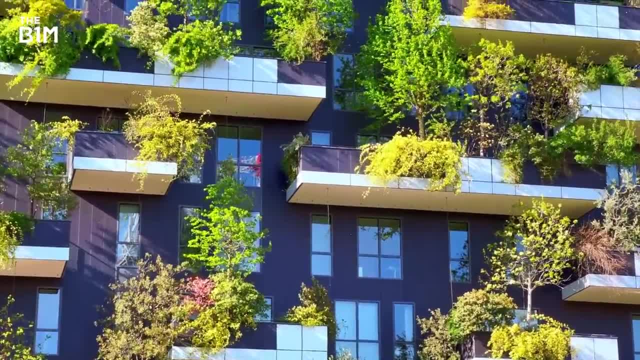 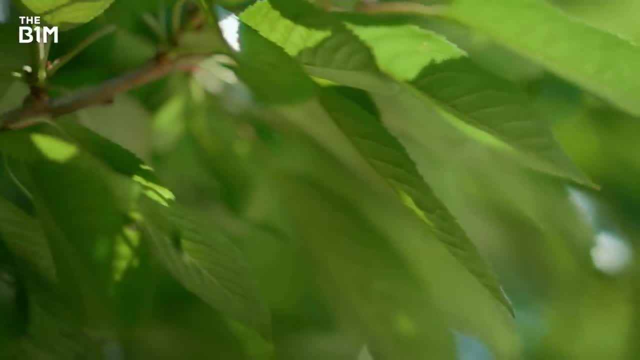 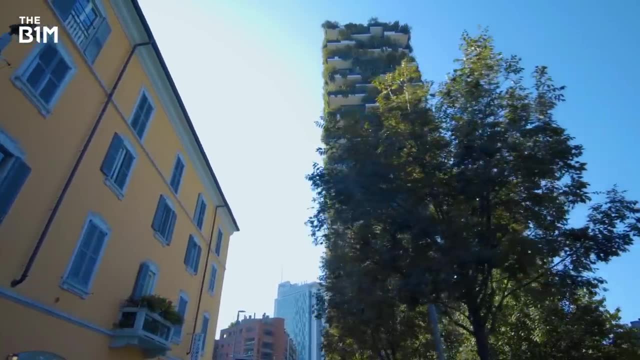 According to the architects, it provides a habitat for over 1,600 bird and butterfly species, though that in itself does create a maintenance issue. It's also not just an upgraded structure that buildings like this need to think about To prevent water getting inside. Bosco, Verticale and green roofs in general have a water-resistant. 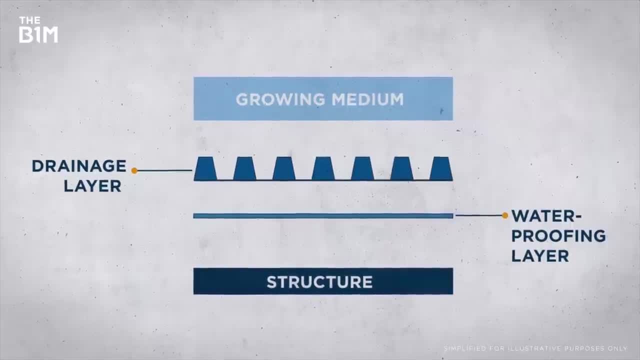 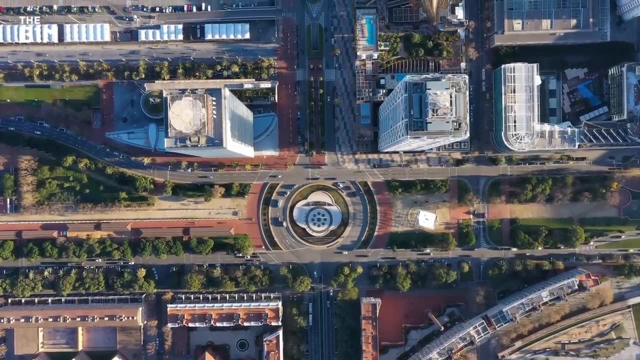 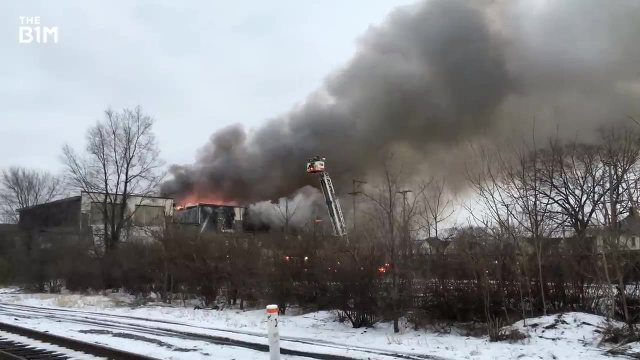 structure, waterproofing and drainage layer between the growing medium and the structure. Fire is another critical area. Many national building codes demand that designers and engineers prevent fire from being able to spread up a building through its external cladding or facade, or to design systems that 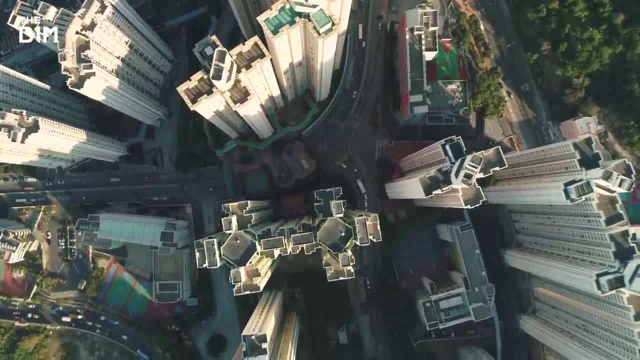 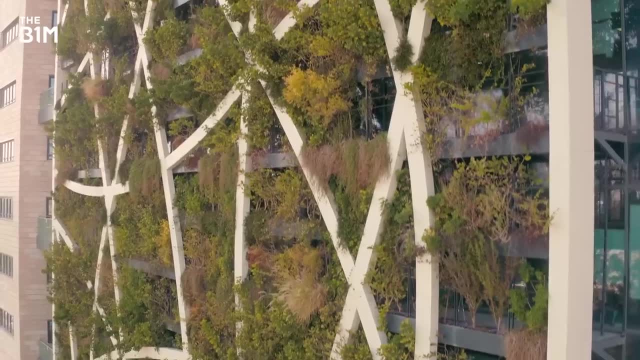 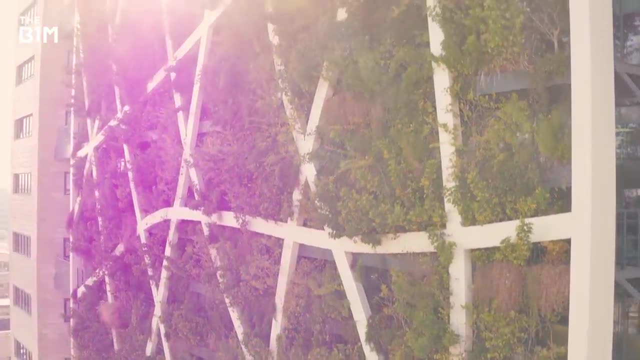 protect occupants and the structure's overall integrity. should that happen, Any plants or trees need to be added and then maintained to meet those specific national rules. Typically, that means keeping them to a certain size, preventing them from becoming too dry and incorporating the right fire suppression and evacuation systems. 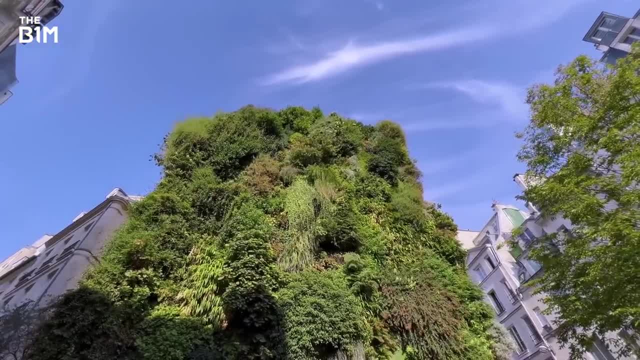 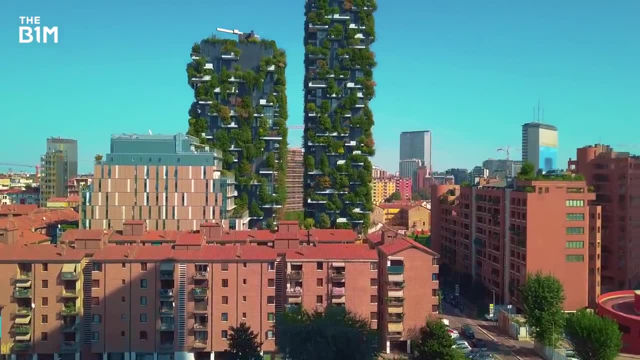 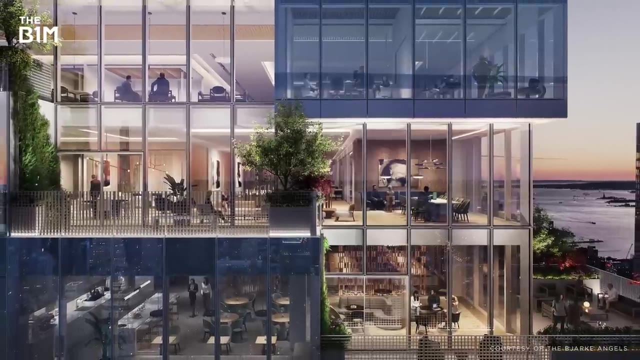 Despite the touted benefits of adding trees to our buildings, it's perhaps telling that we haven't seen an explosion of fully completed projects looking just like Bosco Versa Cale. In fact, very few structures have even tried to come close. The Spiral in New York was pitched as a lush addition to the concrete jungle, but now that 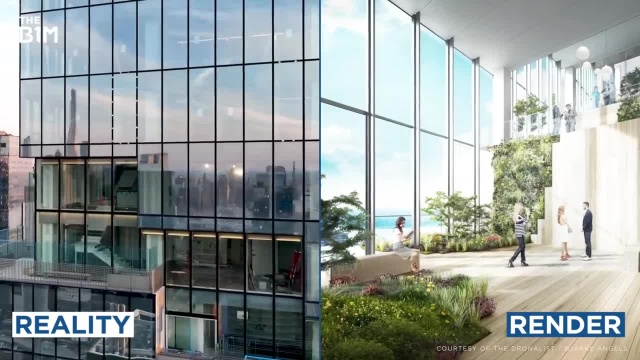 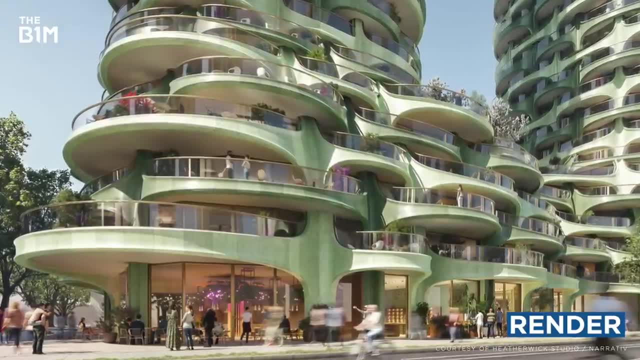 it's complete. it's greenery free. It feels like a far cry from the renders – though, granted, it's still early days. Many other projects go for a sprinkling of trees rather than attempting a full-blown forest, and the finished results can often end up a long way from what was shown in the. 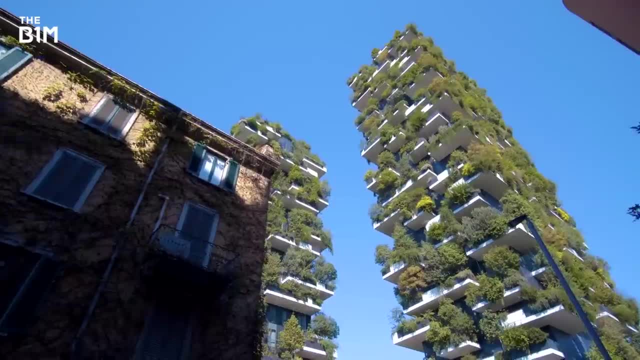 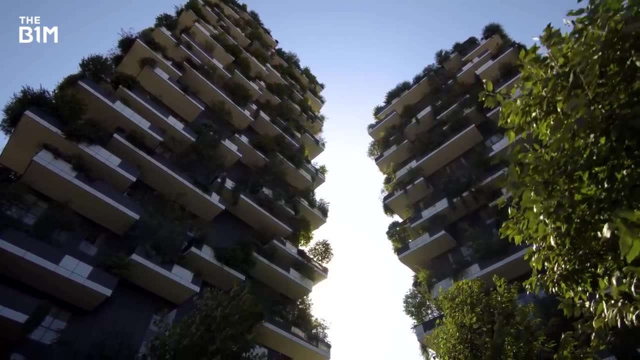 design renders. But it's not just other projects falling short. Some believe that Bosco Versa Cale feels like a standout anomaly because it had a helping hand. The real project gets built right before the Milan Expo, So it's like the government is helping. 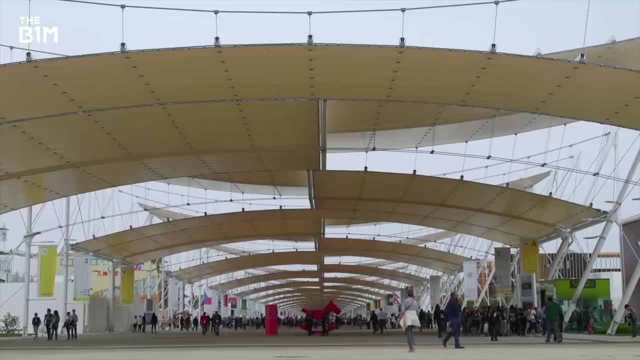 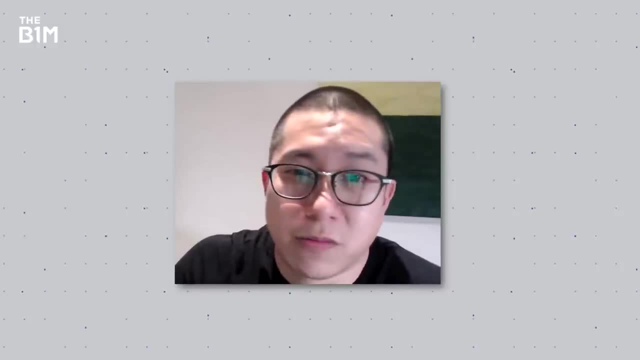 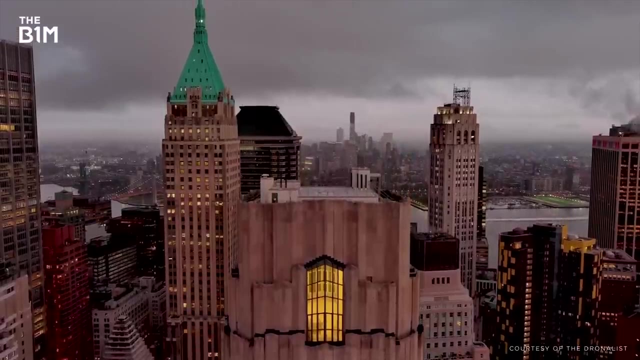 They have that project as a showcase project for the city, and that doesn't happen all the time. These kind of projects all have legal challenges that you have to go over, like the code issues because you haven't seen it before When it comes to, let's say, New York or cities that have long history and code issues. 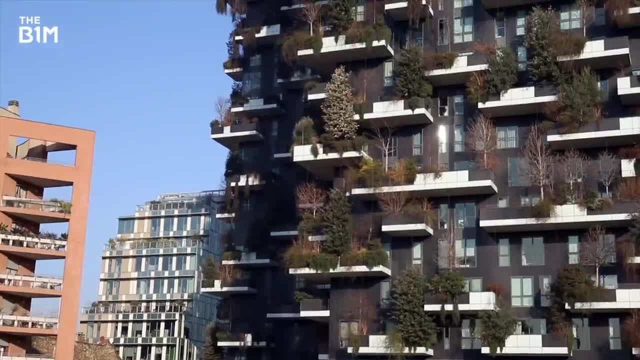 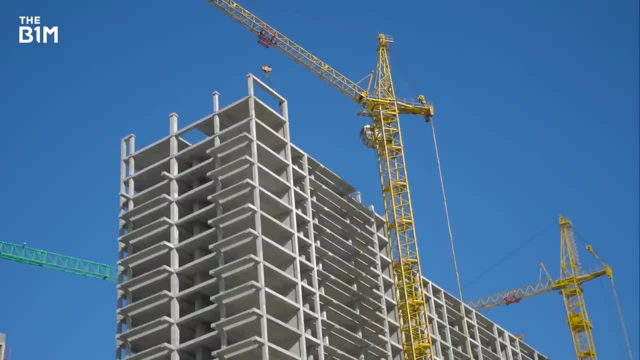 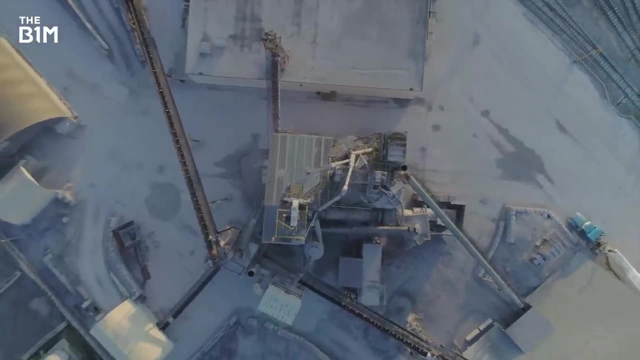 then it's a whole other game. As you might be gathering, adding trees isn't a stroll through the park. Balconies need an immense amount of concrete. That means stronger foundations and superstructures and extra cost. On top of all that, concrete production is a huge source of CO2.. 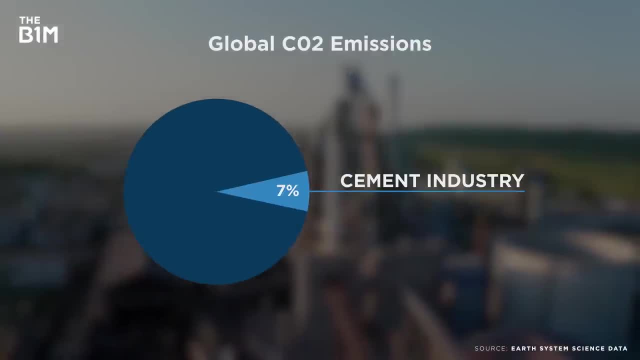 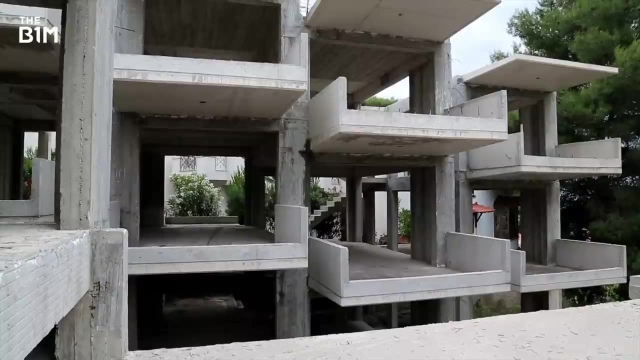 In 2021, the cement industry accounted for 7% of all global emissions. So while extra trees in an urban environment may reduce carbon over time, the concrete can actually add to it. in the initial construction phase, Steel isn't much better. 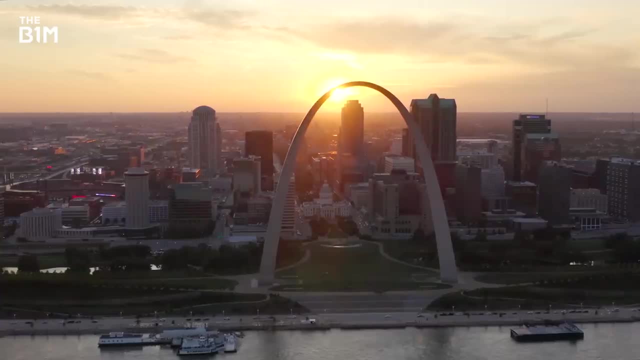 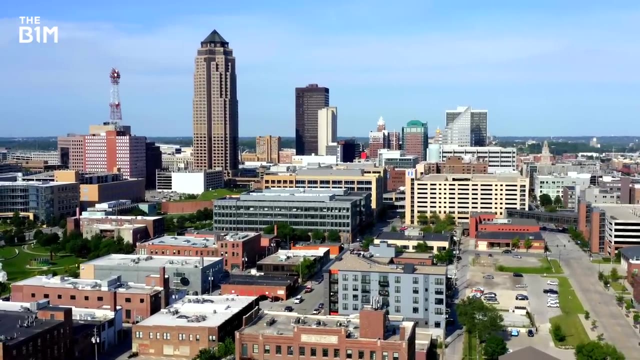 There's also significant long-term maintenance to be done. There's also significant long-term maintenance Both for upkeep and safety and those added fire considerations, All of which again adds more capital and operating cost. For some, it feels like just adding a few trees at the render stage is a move to win. 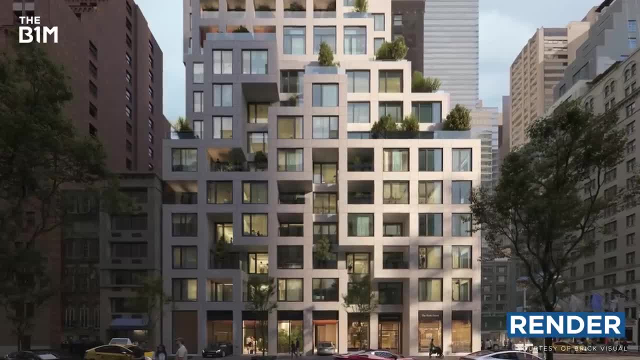 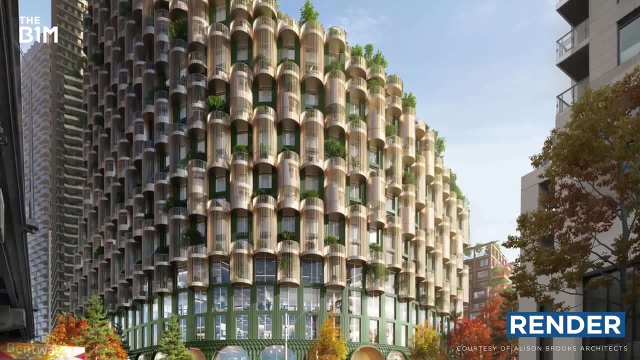 over planners, reassure local communities, close real estate deals and get your Instagram like count up, And that's an important bit of context. Many new projects need public and commercial support in their early stages, and ensuring a good reception to your renders in the first place is key.